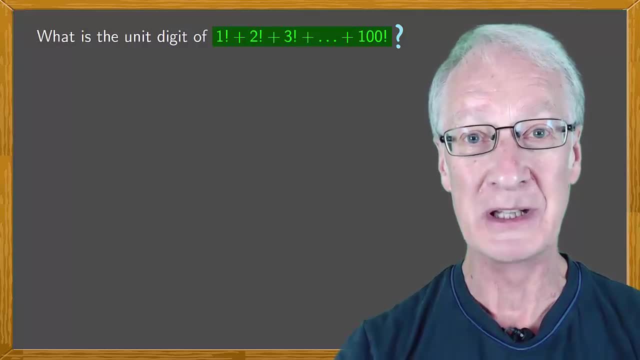 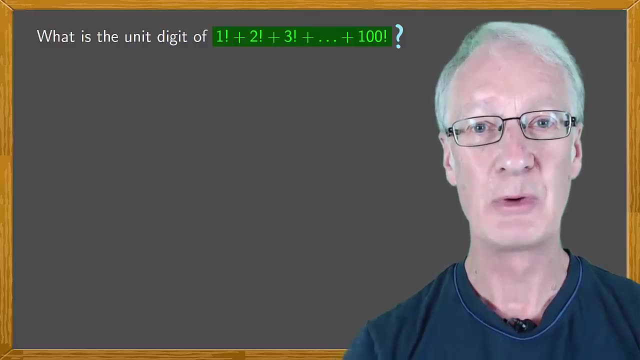 But very obviously that would take a long time, It would be very, very laborious and in any case there is a much better way We can calculate the first few sums and see if we can deduce a rule or an expression that gives us the last digit without having to work our way through the whole calculation. 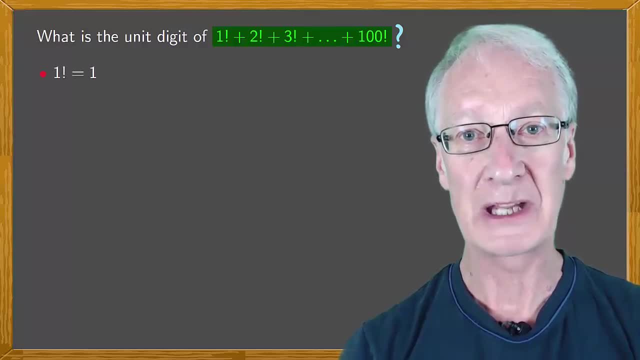 First of all, one factorial is one. Now, if we calculate one factorial plus two factorial, this is one plus two, which is three. Continue: One factorial plus two. factorial plus three. factorial is one plus two plus six, that's nine. 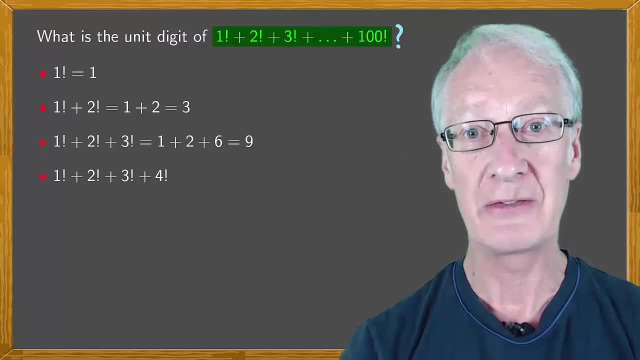 Next, one factorial plus two factorial plus three factorial plus four factorial is nine plus four factorial, which is four times three factorial, or four times six, which is twenty-four. No doubt you're making a bit of a fuss here. You shouldn't. 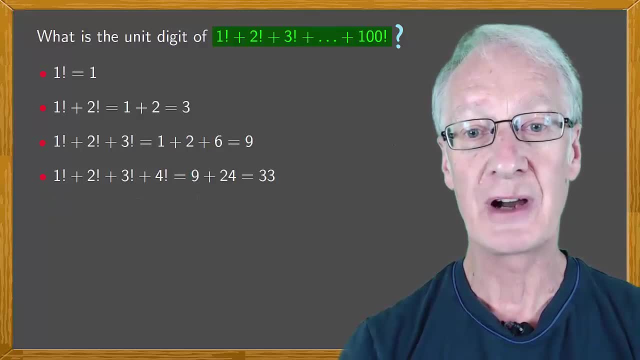 is 33.. Well, so far our last digits have been 1, 3, 9 and 3, and it's hard to see any pattern emerging yet. So moving on to 1 factorial plus 2 factorial plus 3. factorial plus 4. factorial plus 5 factorial is the previous result, 33 plus. 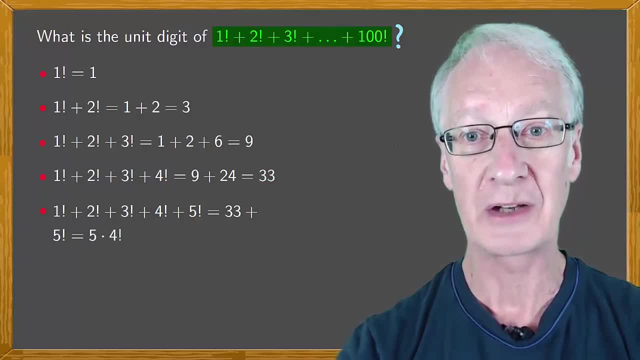 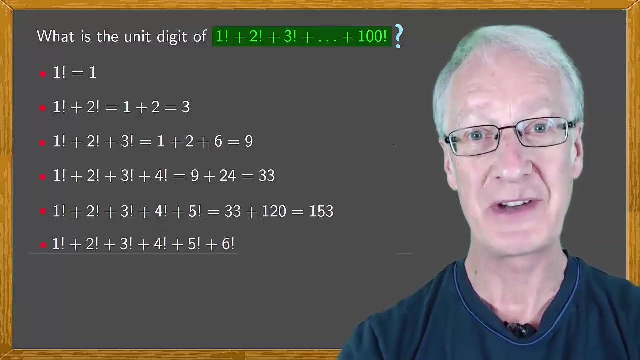 5 factorial, which is 5 times 4 factorial, or 5 times 24 or 120. so we have 33 plus 120, which is 153.. Now can you see a pattern? Well, we'll do one more step and then you'll see it for sure. Next up is 1 factorial plus 2 factorial plus 3. 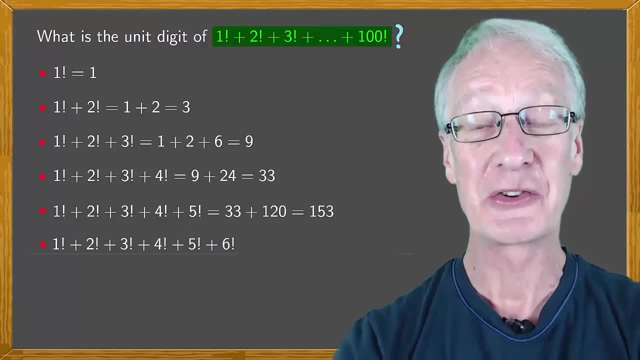 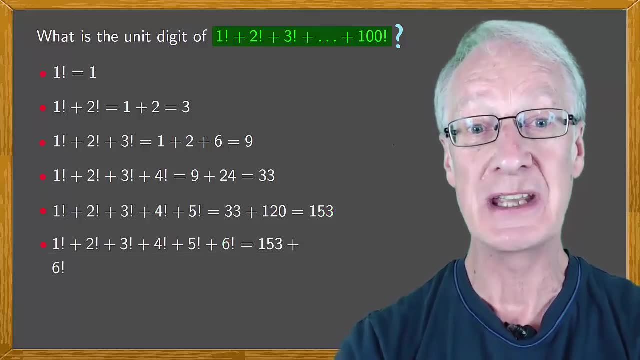 factorial plus 4 factorial plus 5 factorial plus 6 factorial, which is 1 factorial plus 3 factorial plus 4 factorial plus 5 factorial plus 6 factorial, which is the previous result, 153 plus 6 factorial, which is 6 times 5 factorial, or 6 times. 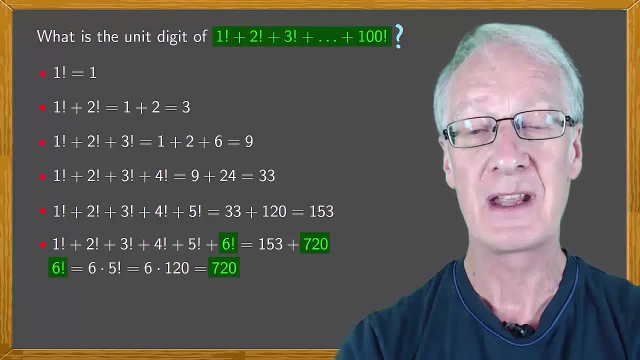 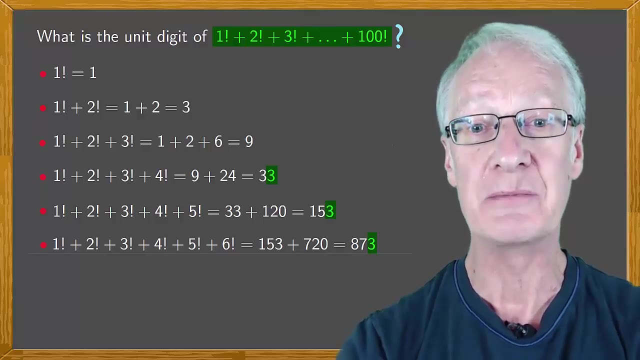 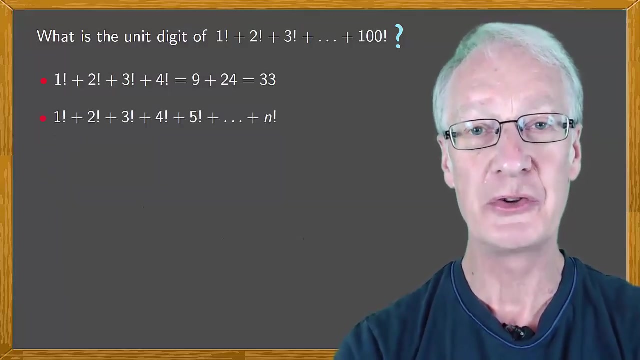 120, which is 720, and 153 plus 720 is 873.. Notice that in the last 3 results the final digit has been 3.. Is 3 always going to be the unit digit from now on? Notice that in general, for any sum, 1 factorial plus 2 factorial plus 3.